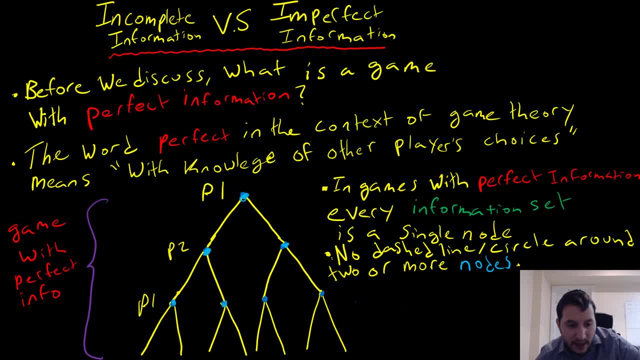 in a lighter blue. Those are information sets and they are singletons here, And what that means is that there is no information set with two or more nodes, So we don't have any dashed line or circle. So we have none of this stuff here. None of you know this stuff here, Right? None of that. So it's just really- let me clean this up a little bit- Just a game where you know. 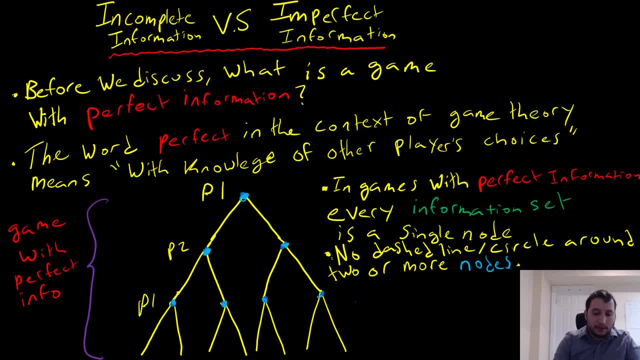 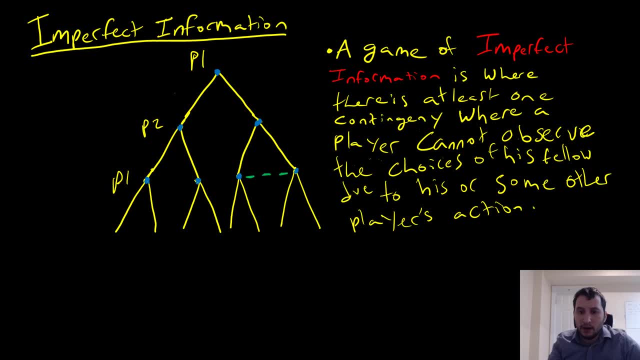 every point where you are on the game, Moving on a game of imperfect information, is where there is at least one contingency where a player cannot observe the choices of his fellow due to his or some other player's action. So this is illustrated just in this game here, where we have a information set down here. So if player one goes and chooses this choice here, so this is going to be. 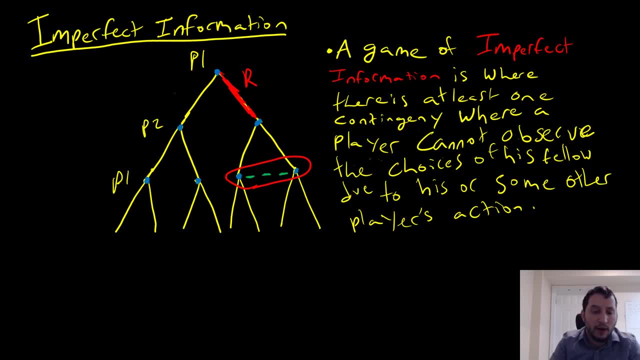 right, I didn't go and label this so well, just to go and communicate that the main focus is on the information sets. So that's just to go and clarify that. But if he moves right here, what we're going to see is that player one is going to be essentially throwing himself in the dark and player two is able to move. So what player one is doing is that he's moving himself effectively into a simultaneous move game. Just you know, remember. we can equivalently write this: 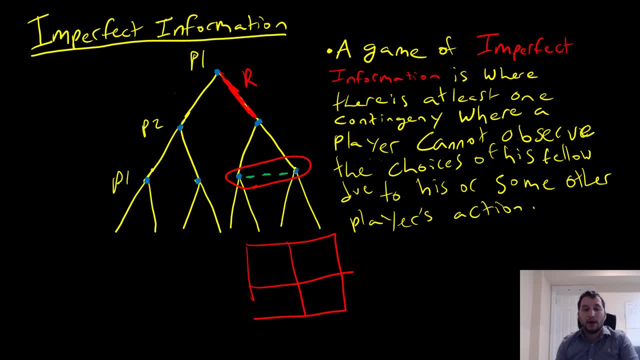 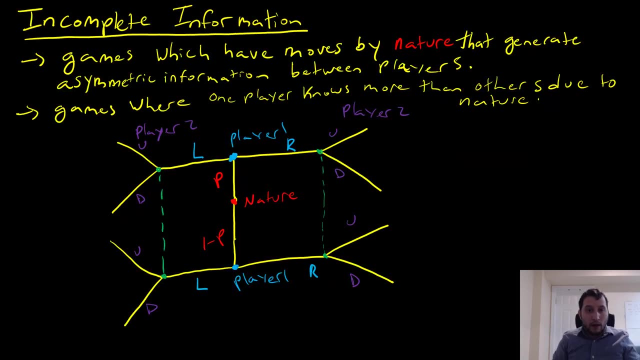 as you know, as some simultaneous move game right over there. Basically, if you see an information set around a player's actions right- and we're going to use this word player right- it is a game of imperfect information. Now, the word incomplete information means that we have a move by a player named nature and it generates asymmetric information between players right And 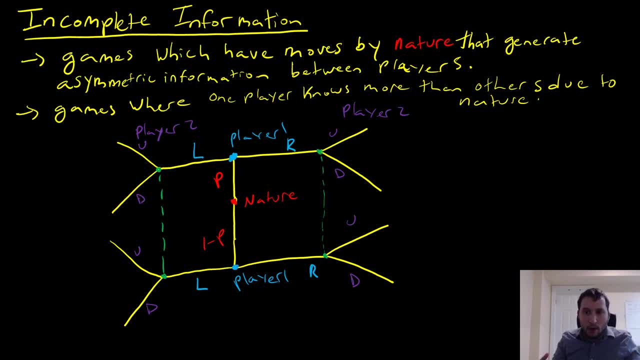 this is a game where one player knows a lot more than the other player does. So if you have a setup like this one, this is like a beer quiche sort of setup: right that you go and you have here right, But nature, right, it is viewed as a chance node right And it goes, and it gives player one information about his type. Player two, though, is kept in the dark over here, So